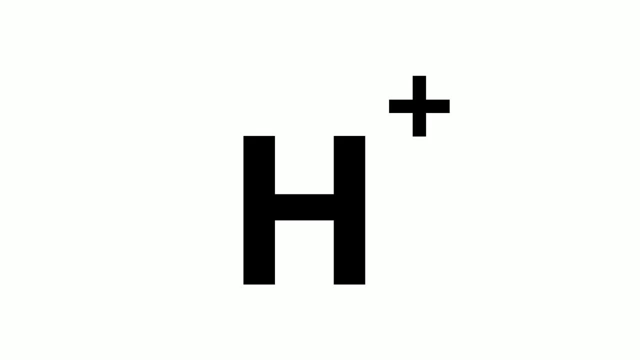 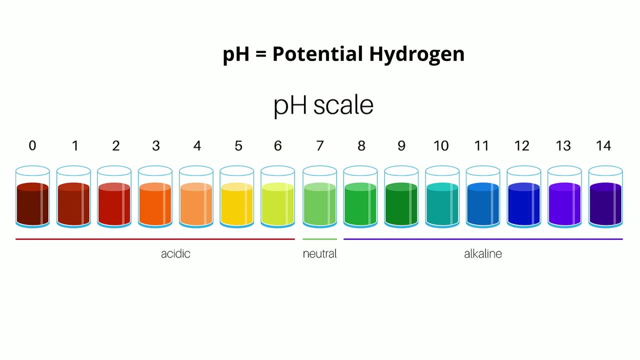 The acidity of a solution is measured by its number of hydrogen ions. You can look up this measure on a pH scale. The abbreviation pH stands for potential hydrogen and it's a measure of how 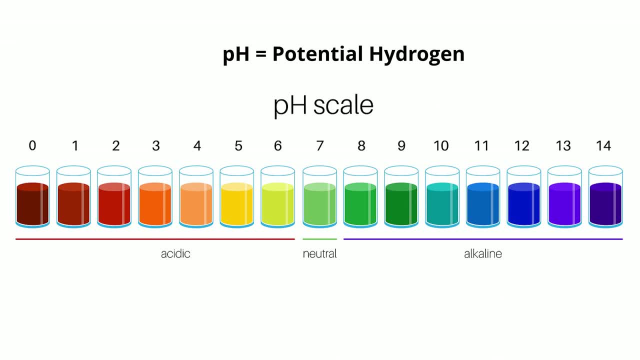 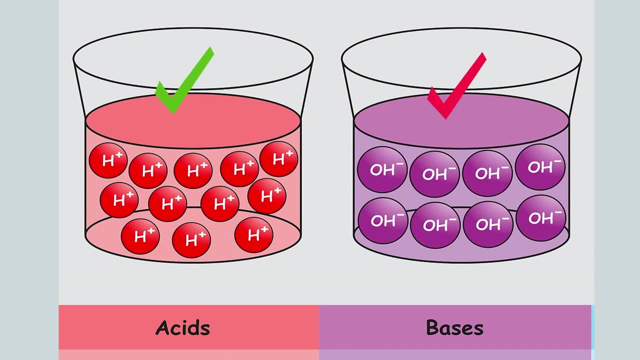 much hydrogen is in the solution and how active the hydrogen ion is. Hydrogen ions determine whether a solution is an acid or a base. A base that is water soluble is called an alkali. 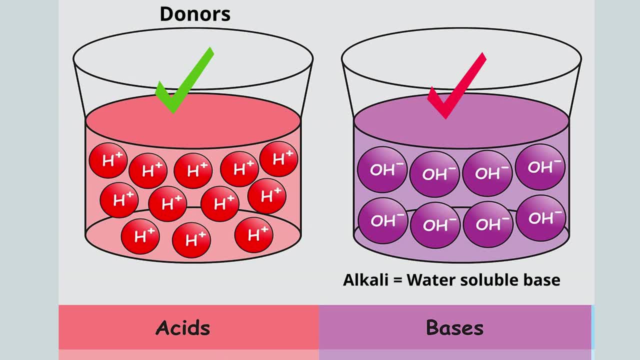 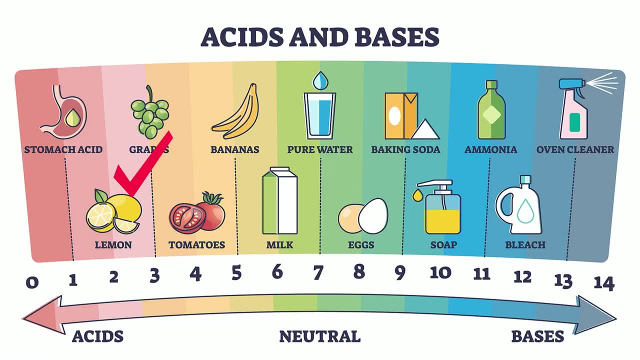 Acids are hydrogen ion donors and alkalis are hydrogen receptors. A substance with a pH lower than 7 is considered acidic and greater than 7 is an alkali. 7 is neutral. Each interval on the pH scale is a 10-fold increase. So a solution with a pH of 5 is 10 times the pH of a solution. 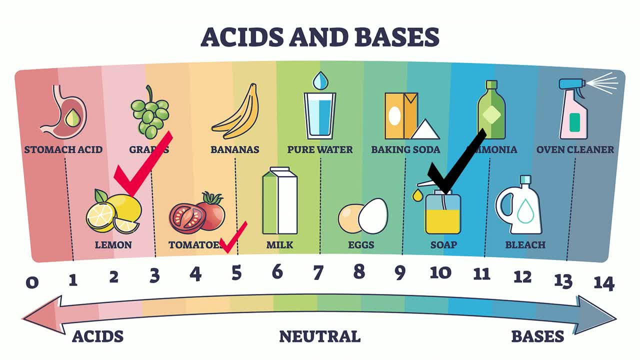 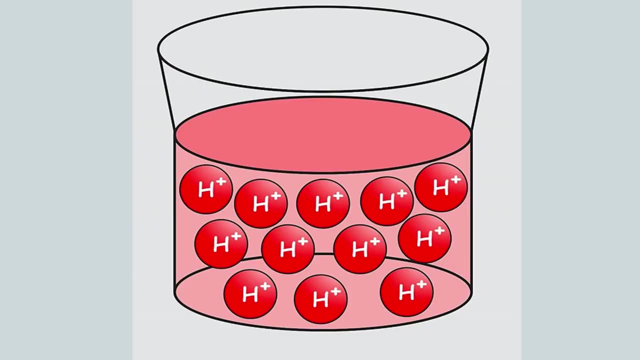 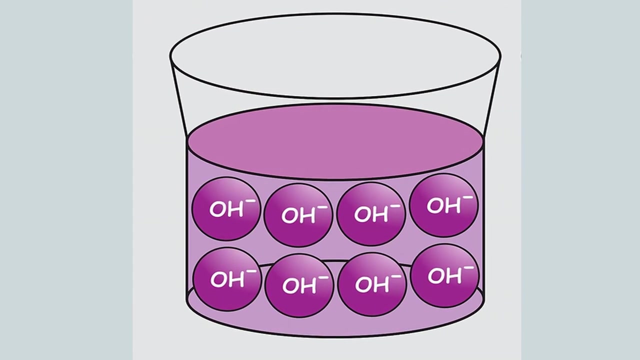 More acidic than an object with a pH of 6. The difference between an acid and a base comes down to the number of positively charged hydrogen ions. When an acidic substance is dissolved in water it releases hydrogen ions causing an increased proportion of positively charged ions. When an alkali substance dissolves in water it releases negatively charged particles called hydroxide ions. Remember an alkali is a base. 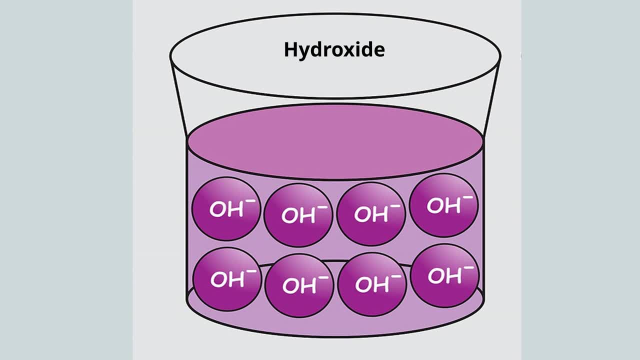 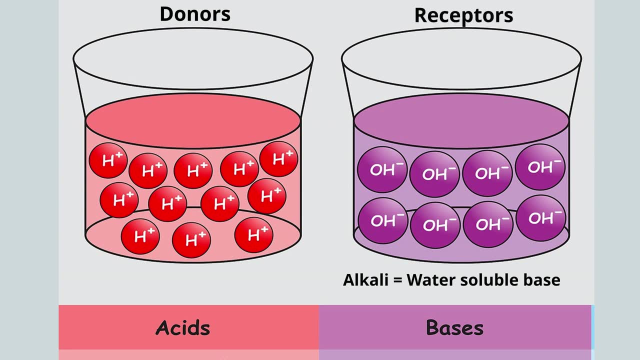 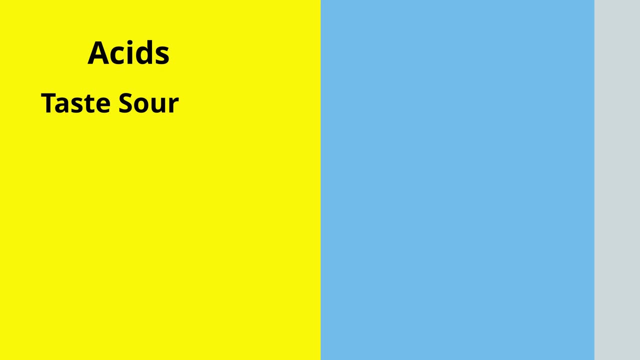 That is water soluble. Again acids are called hydrogen ion donors and bases are hydrogen ion receptors. Let's look at a couple characteristics of acids. Acids taste sour. Acids turn blue 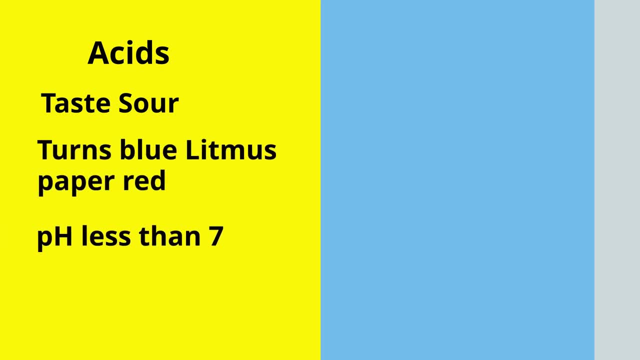 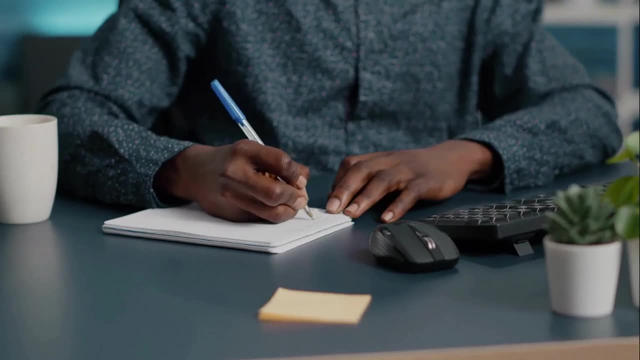 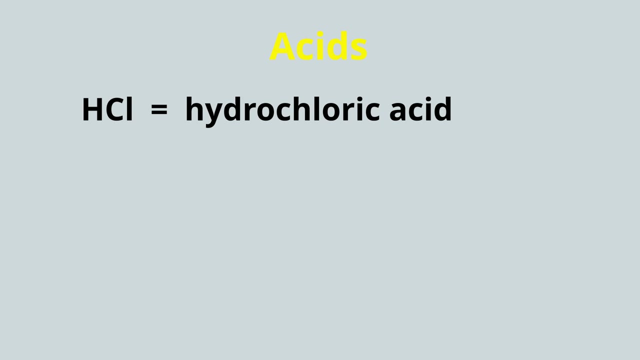 7. Acids typically have a hydrogen in front of it with their chemical formula. HCl is hydrochloric acid. HF is hydrofluoric acid. And bases typically have a hydroxide ion. NaOH is